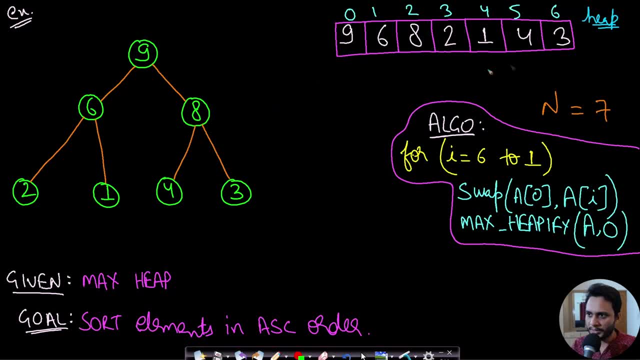 ascending or descending order. then we want to build a heap. okay, we want to apply the build heap algorithm which i have already explained, and using that algorithm you can build a max heap or min heap. and then you can apply this heap sort algorithm. right, so heap sort will be making use. 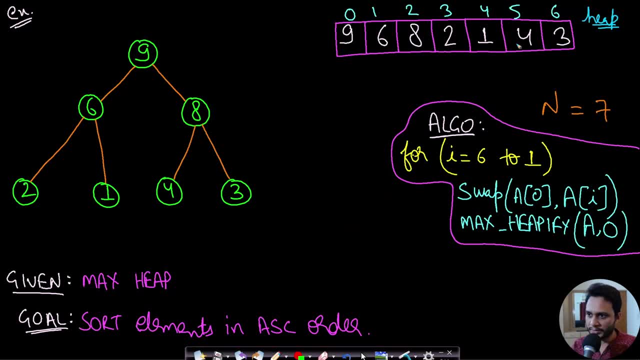 of build heap. first, let's assume that we are given a heap, because i have already explained how to implement build heap algorithm in my previous videos. link for that will also be present in the description below. now, in this case, if this is a max heap, given a max heap, we are required to. 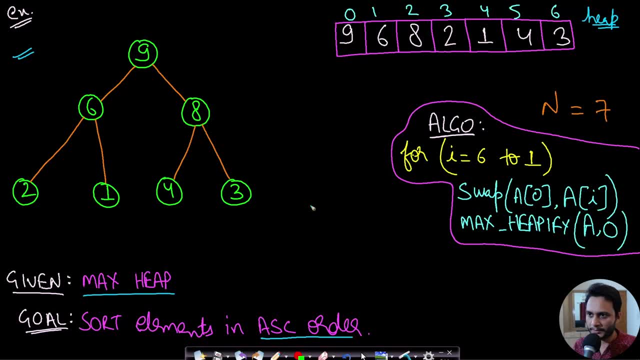 sort the elements in, let's say, ascending order, then how do we do that? now? in this case, the algorithm says that first we will be building a heap, so let's assume that this is a max heap already. we know that this is a max heap. then after that, what we do is we will have to extract the maximum element. now how? 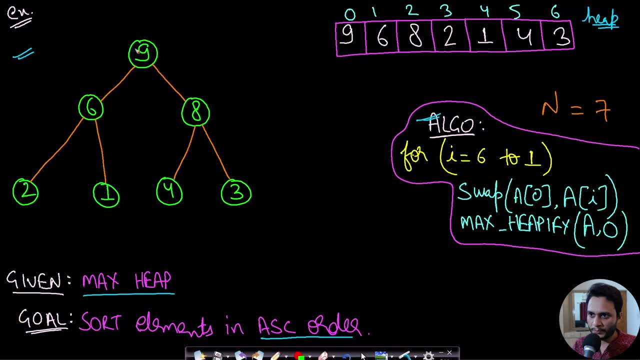 do we extract the maximum element? i have already explained it. what we will do is we will copy this maximum element somewhere. let's say we take a max variable, we copy it nine. okay, now the next step is we will take this last element and we will copy it to the root and we will remove this link. 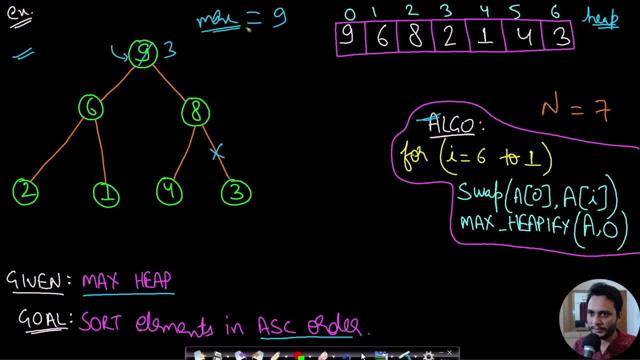 so what operations are we doing? we are storing the maximum element in max variable. we are copying the last element in the first element. so this last element in array three is copied to the first element. so this will become three. right, and now the last link is broken. that means the heap size. 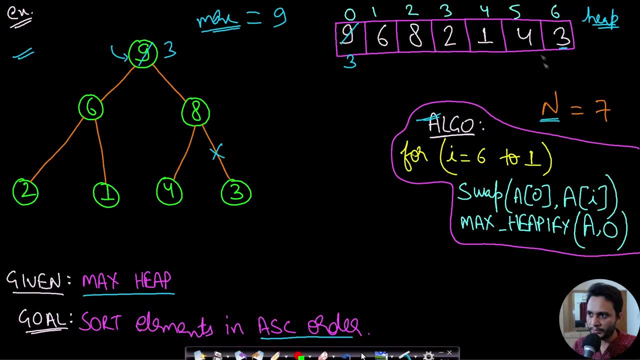 is reduced. so let's assume that our initial number of elements were seven. so now, since we are reducing the heap size, it will be six. okay, and after that we will be copying this max element to the last element, so this will become nine, and now we will be max heapifying the root because we want to. 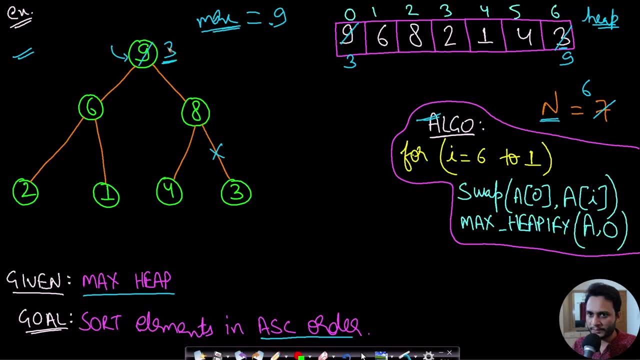 maintain the maxi property. so if we max heapify this one, then this is three. maximum of left and right is eight, so eight will come here. three will come here again. maximum of left is four, so right will not be taken. because we have removed this link. we have decreased the heap size. it is now: 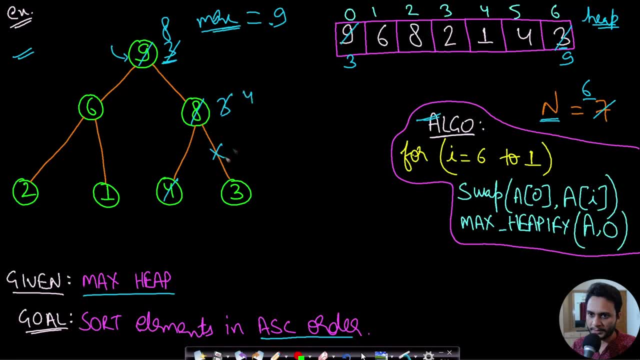 six. so that is why, uh, four will be replaced here and three will come here. right, so this is after sorting one iteration. so we will be iterating for all the n minus one elements, because let's say we have n elements and if we can sort n minus one element, then obviously the last element will also. 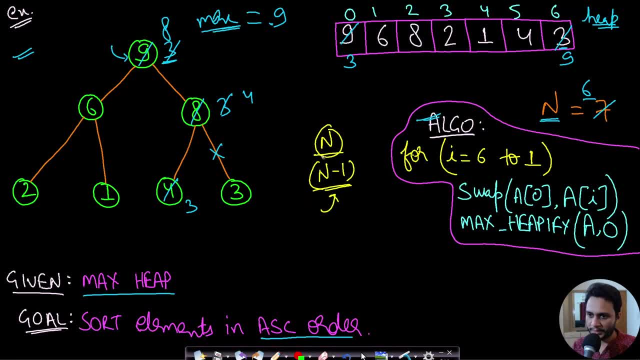 be at the correct position. it will also be in the sorted order. so if we are given an elements, we will be sorting n minus one element. in this case we were given seven elements, so we will be sorting six elements only from six to one right. so we have sorted one element. maximum is pushed to the right. 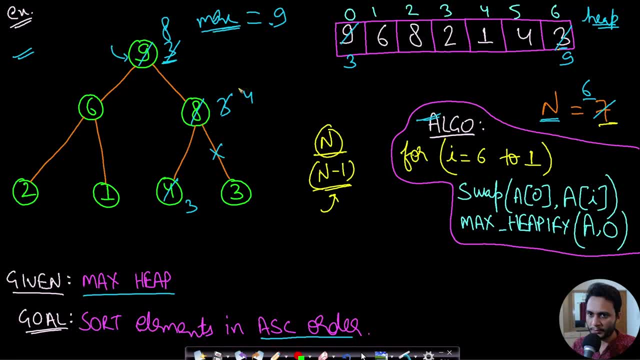 hand side, that is the rightmost element, is the maximum element. now what we will do now? heap size has been reduced by one, so now eight is the root. okay, so now we will again repeat the process with the extract Max. so now we will again extract the maximum element. this Max variable will be storing. 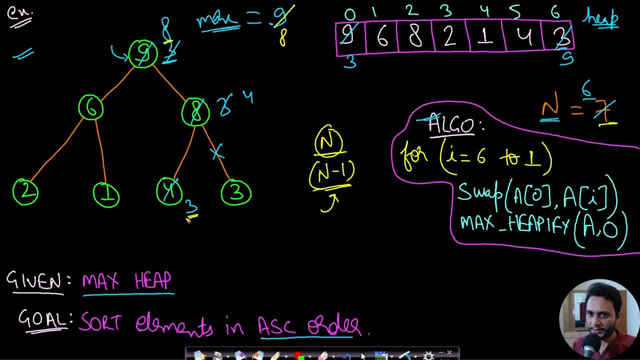 eight, okay, and now the last element here is three. so three will be copied here. okay, and now eight will be moved to the last element of the heap, because heap size has been reduced by one. so last element is this: four. so or eight will go here. right now we will apply the. 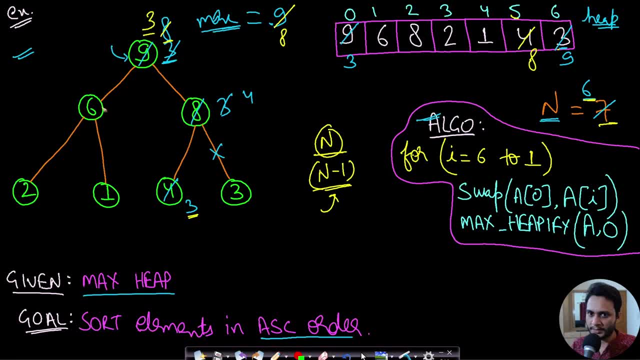 max epify on this: three, so maximum of six, and four is six, so six will come here and three will go here again. three is maximum among the left and right child, so it will stay here and max epify is done. okay, now, once we are done with the max epify, we will be decreasing the heap size. so this link: 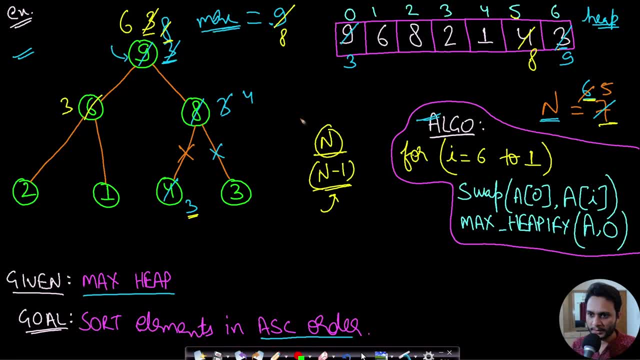 will be gone and the heap size will become five. now, okay, now we will again repeat the process. six is the root. now we will again apply extract Max. so Max will be storing six. last element: what is the last element? last element is one, so one will come here. 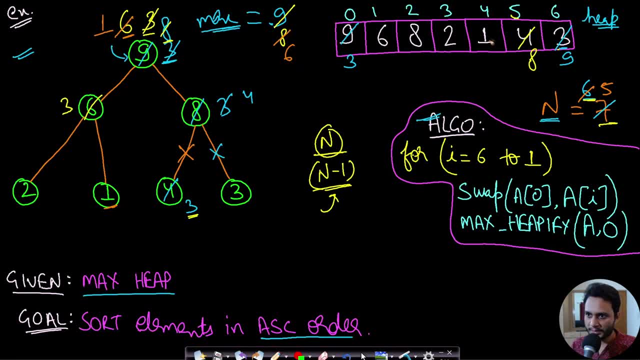 okay, and now six will be copied to the last element. so this will be six and we will apply max epify on this one. if we apply max epify on one, then among the left and right child, which one is maximum? four is maximum. so, uh, four will come here and one will go here again. 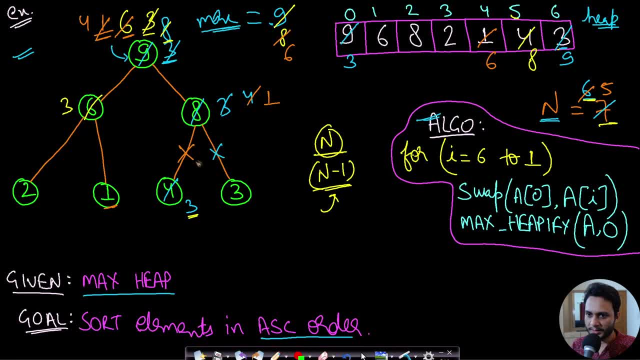 uh, this one is not having left and right shared because the links have been removed, right, so this will stay at this position. this is a leaf node, and so max epify is done. so now we have sorted three elements, and so, uh, this link will also be gone, right, so the n value will now become four. so when? 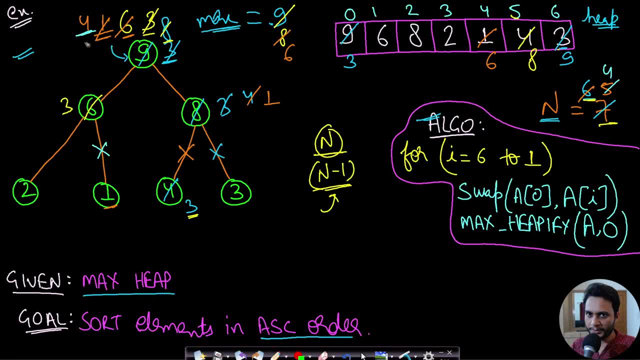 the n value is four. again, the root node is four. so we will again apply the extract Max algorithm. so extract Max, uh, this will store four and and the last element is two. so two will come here, okay, and this four will be copied to the last element because heap size is four. now, right, and again we will apply max epify on this two. so if 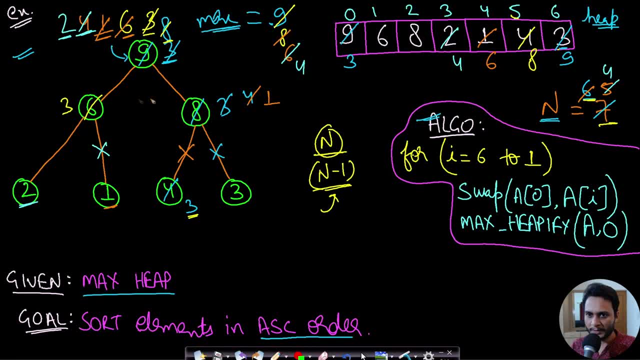 we max epify this two, uh, then maximum of left and right is three. so three will come here and two will come here right, and since this is two, I mean this link is gone because you have already considered this one. so now we will stop max epifying right. so actually, uh, 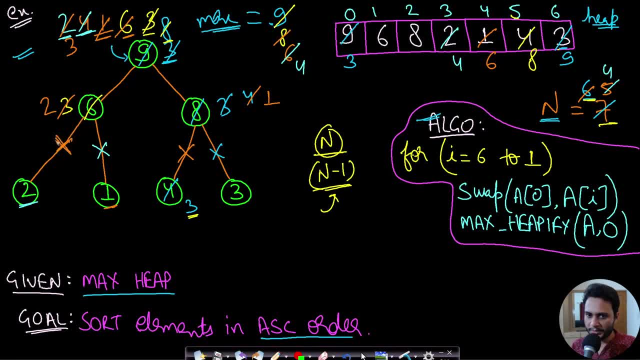 this link should have been removed first before doing the max epify. this you should remember. so now we have max epified four elements right and this n value will now decrease to three. so if you look at the tree, then let me draw it, redraw it. so three is here, two is the left child. 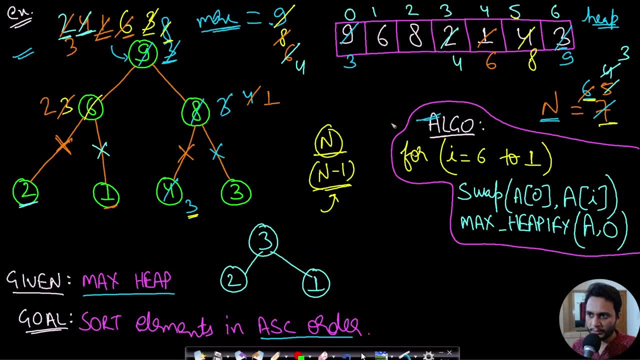 and one is the right child. okay, so if you keep applying this algorithm like a heap, size is three now, so maximum variable was storing four. now again you apply extract Max, so this will be storing value three. right, and since this is storing value three, it will be. 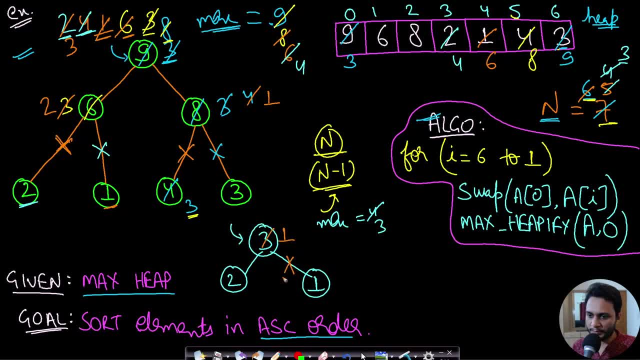 replaced with the last value. so one will come here. you will have to remove this link first and then apply max epify. so apply max epify on this. if you apply max epify, then two will come here and one will go here. so what was the max value? it was three. so three will be copied here. 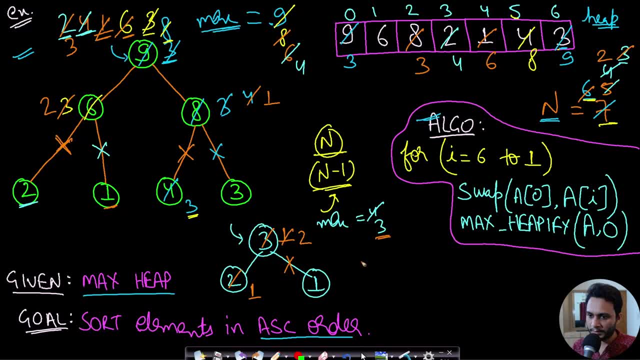 right, and the heap size will become two. now. now the heap is having just two elements. this is root one. okay, now again, you apply max extract Max on this one. so if you do that, then this is maximum. so maximum will now be storing two. one will be replacing the root element right and this link. 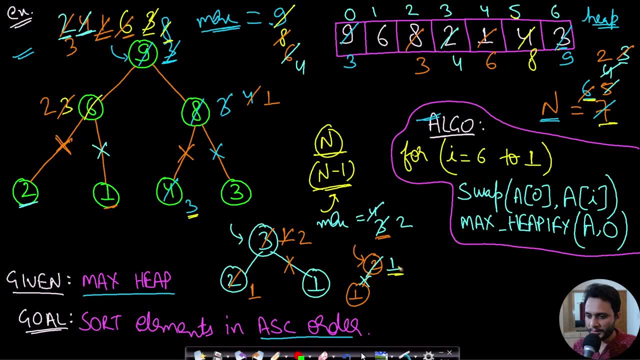 will be gone and after that you will have to again apply max epify. but this is the only element, so this will always be in a maxi forum in here format. I have already explained this, so no need to do anything now. you will copy two here, right and so. 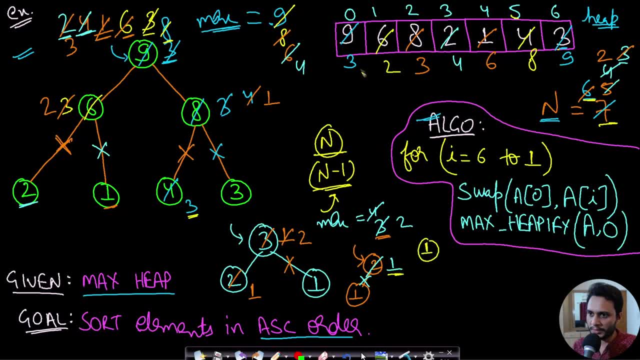 uh, you will be having just a single element, which is one, so one will by default, be at the first position. okay, so I have not shown you the changes for this zeroth index. actually, whenever we were swapping the elements with the rust element, then this zeroth index value should have changed, okay. 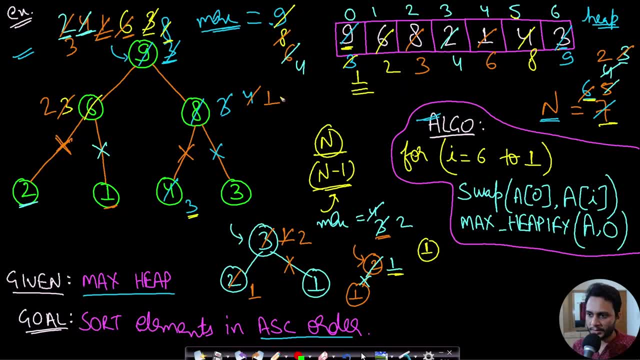 so I hope you understood the entire algorithm right. so this is nothing but a combination of extract Max algorithm, epify algorithm and build heap algorithm, right? so if you want to sort a heap, then an array may or may not be a heap, so first you will apply build heap algorithm. it will. 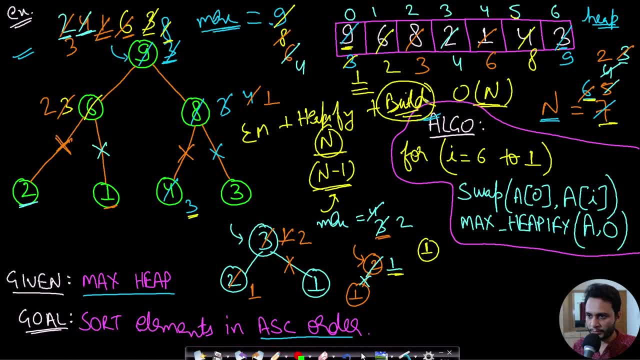 take order of n time after building a heap. let's say you build a max heap, you will have to apply extract Max for n minus one elements if you have n elements and for each element you will have to again apply epify for the root element, right? so epification will take maximum of order of log n. 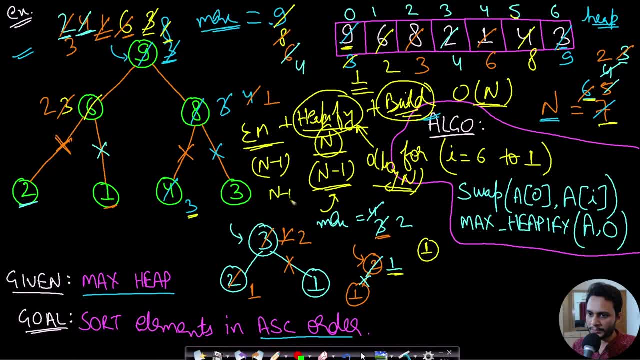 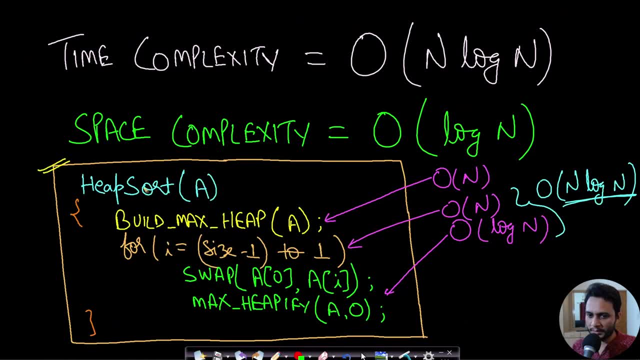 time right, and you are doing it for n minus one times. so the total time complexity will be n log n. now let us look at the algorithm. this is the entire algorithm here. this is the heap sort where we are sending an array. so this is nothing but an array. so once you have sent an array, then 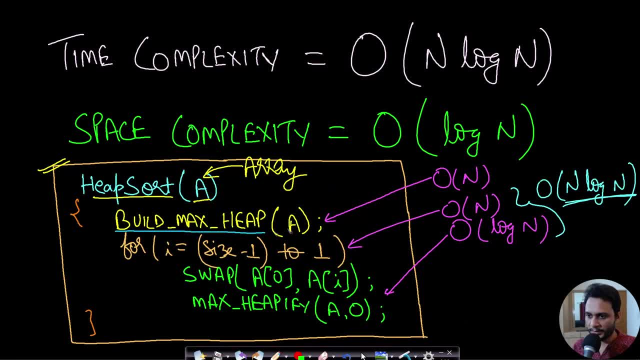 it may or may not be a heap. you will have to build a heap out of it. building a heap takes order of n time. now, once you have built a heap, then if it has n elements, then we will be extracting n minus one maximum elements. okay, so we will be running from size minus one to one. okay, if you have size. 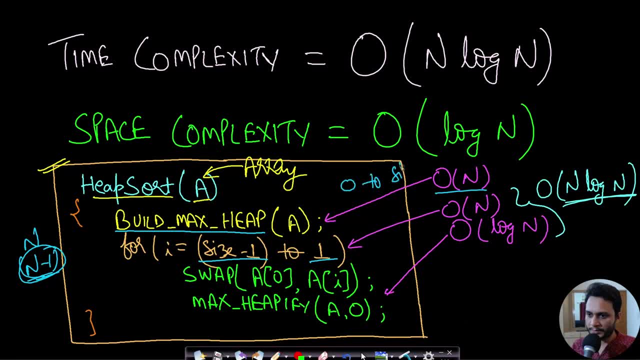 of elements and if it is zero index from zero to size minus one, then basically we are leaving the zeroth index element and that, and if we extract n minus one elements, the last element will always be sorted right. we will be swapping the root element with the last element. this I had shown. 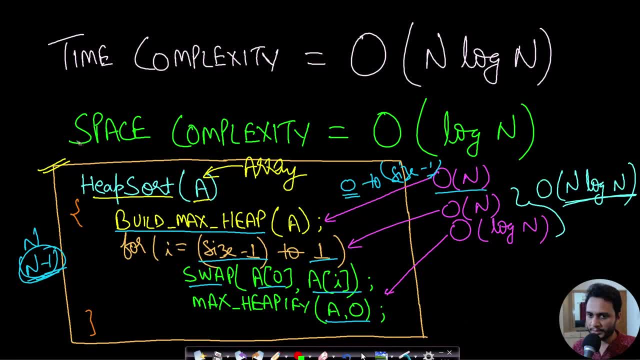 and again apply max epify to the last element. so this is a simple algorithm and here you can see that this loop, this will be running for order of n times- okay, because it is minus one elements and inside that there is a max epify which will be taking log n time. 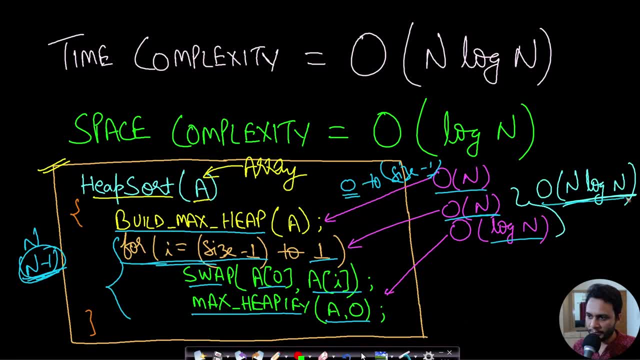 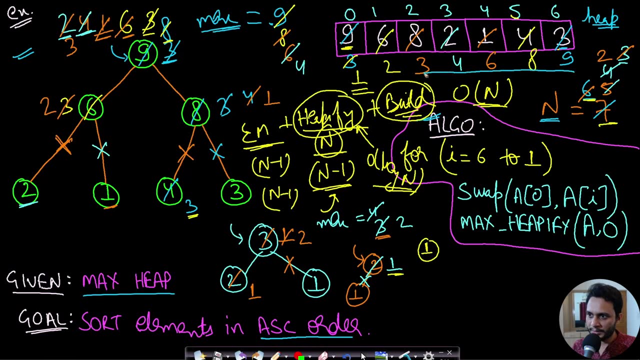 so, since it is nested, therefore, the total time complexity will be: order of n log n, right? I hope you understood this entire algorithm now. if you want to like, arrange it in descending order, like here, I had showed how to make in ascending order. so from the right hand side it is in descending. 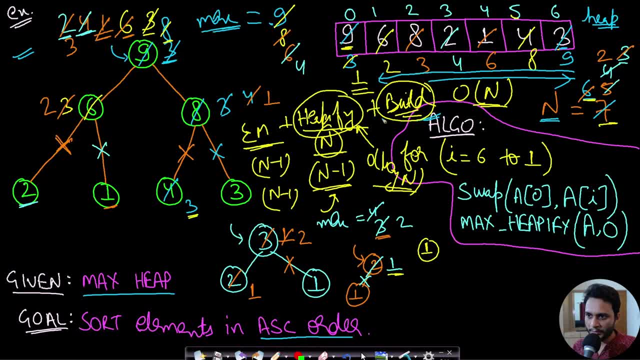 order from the left hand side it is in ascending order okay. so if you want the elements in descending order, you can simply go with the min heap, okay. otherwise you can just reverse this array. both will work, but try to apply min heap. now let us look at the code implementation for heap sort. 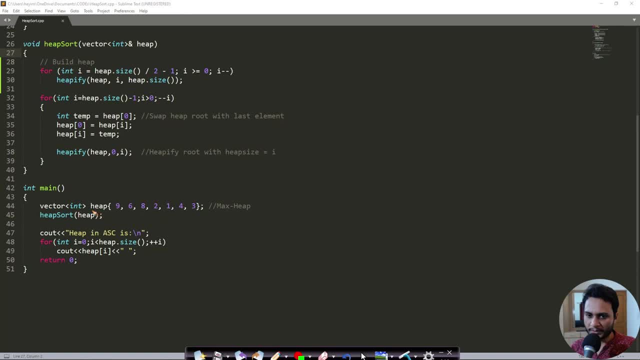 this is a simple code implementation for heap sort. here I have taken an array and the name of the array is heap and I am applying heap sort once the heap has been sorted, then we will be just printing the heap. okay, so let us just see the heap sort here now in this heap sort algorithm, or 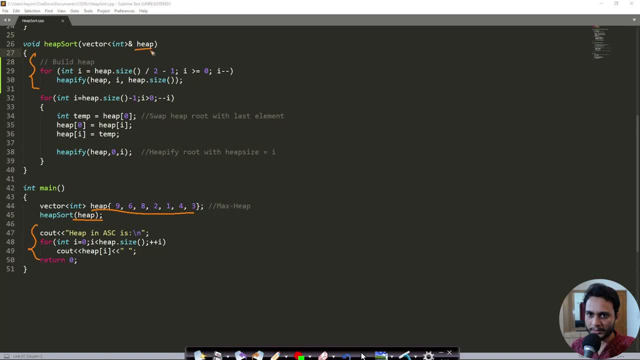 you can see that I am first building a heap, because this may be an array, okay, and if you already know that this is a heap, then you can skip this part entirely. right, this will take order of n time. now, once you know that this is a heap, then we will be applying the extract Max for n minus. 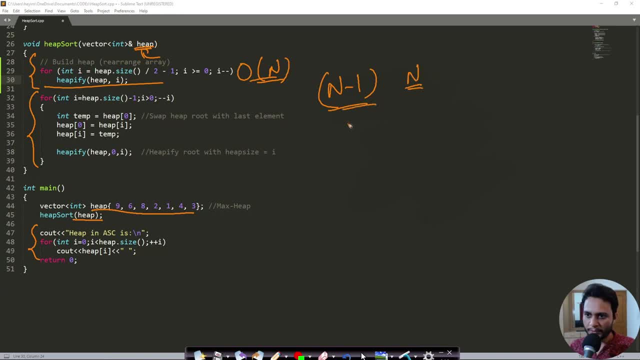 one times if we have n number of elements. okay. so how do we extract? we were actually saving the root element, which was the maximum element, in a temporary variable or a maximum variable, and then we were taking the last element, which is heap at. I heap at, I will always be the last element, okay. 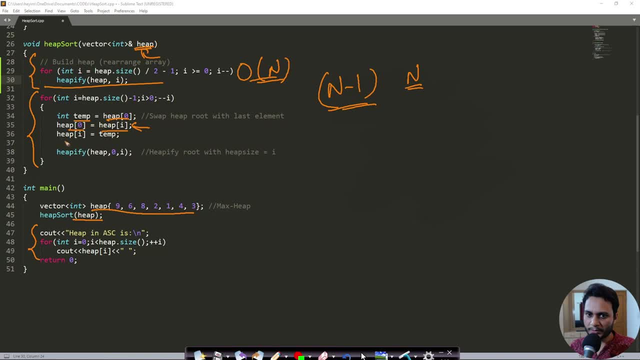 and then we were copying it to the root and once it was copied, then the last element was storing the maximum variable, that is the temporary variable, and then we were applying Max cp5 to the zeroth index element, which is the root. okay, and I is the current size of the heap. so this for loop. 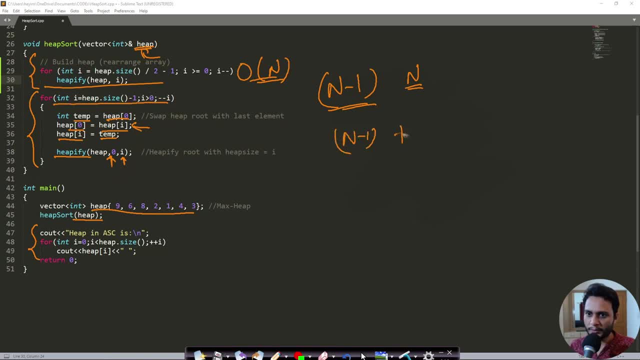 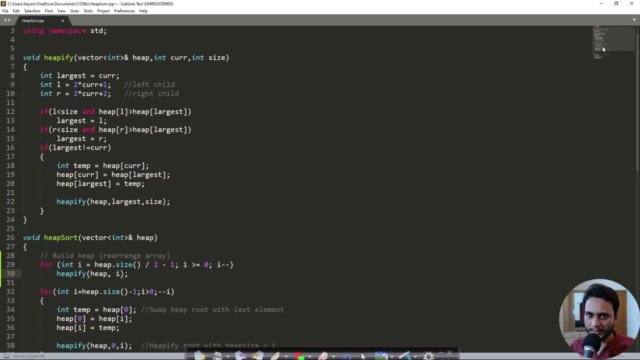 is running for n minus one to one, so the heap size at Max is n minus one because this is zero indexed. okay, so heap size is decreasing by one value for each loop, because once the maximum element is pushed to the last element, then the link is broken, as I had shown in the algorithm. right? so, uh, let us just see the heapify algorithm. 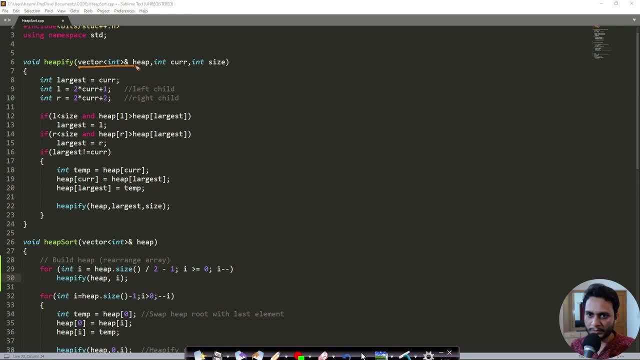 so this is heapify I have not shown you till now. so this is the first video where I am showing heapify algorithm here. it will receive the heap. it will receive the current index, as well as it will receive the size of the heap. now it will take the largest variable. 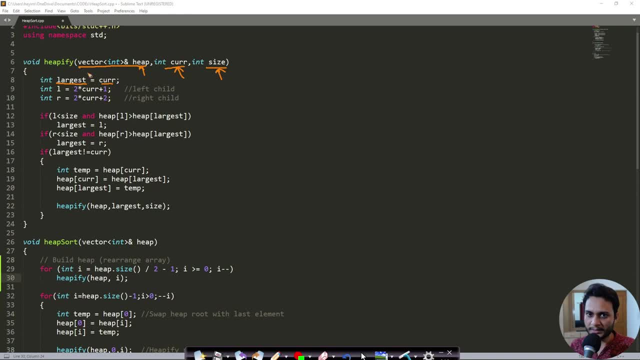 and store the current element, like the current index, as the largest. so this will be the current. okay, now it must be having left as well as it must be having right, so initially largest is equals to this current. now we will check which one is largest. if L is within bounds of this heap size, which is 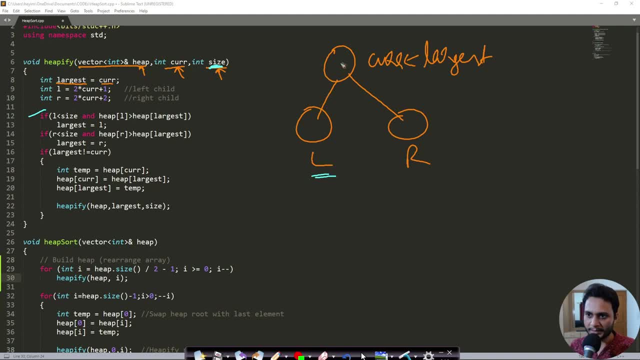 this size and also this L is greater than this root element, then the largest will be updated to L. okay. and similarly, if right is within the bounds of the heap size and also heap at right is greater than whatever is stored at the largest index, then largest will become R. okay. and now if the largest 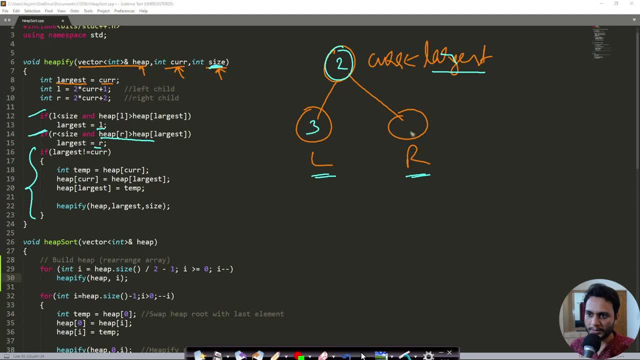 has got changed, like if this was two and this was three and this was four, then at the end of checking all this, the largest value will be storing the index R, okay. otherwise, if this was, let's say, 12, then the largest would have been current only. okay, then in. in that case, we will be stopping the maxip file. 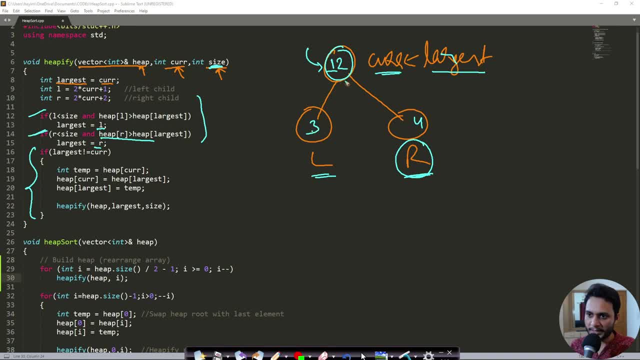 algorithm, as as soon as we find that the left child or the right child, both of them, are lower than this current element- this is the property of maxi. okay, but if you find some index which is larger, that is larger than the current element, then then you will have to again recursively do the HP file algorithm. so let's say it was only two then.